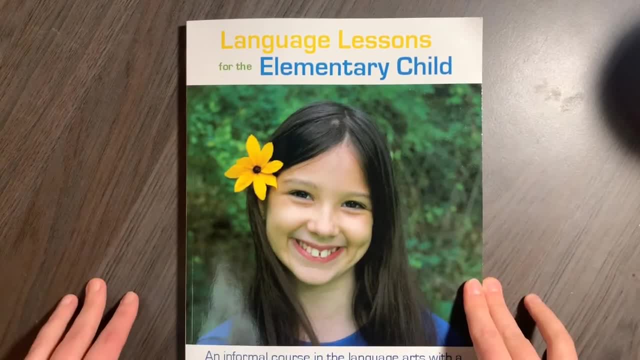 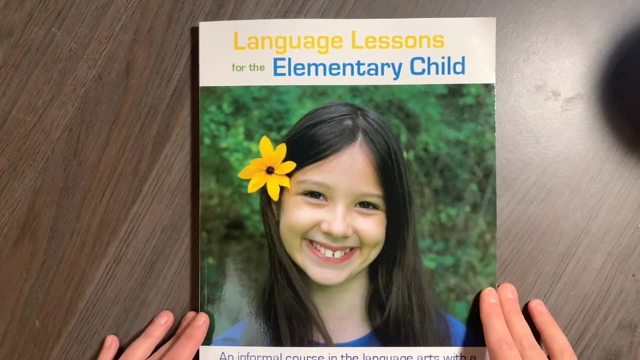 So when I was looking for Charlotte Mason's kind of style language lessons, I was looking at a lot of different curriculums, looking at some flip throughs, looking at some comparisons, And this is the one that I decided would work best for my, my sons, who are right now nine, and they will be 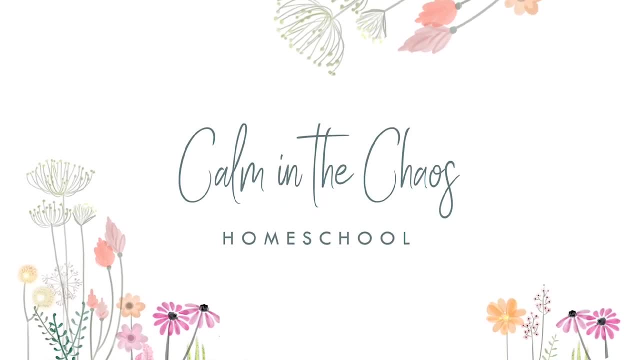 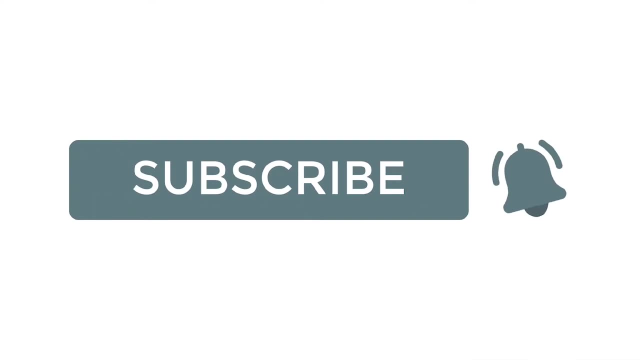 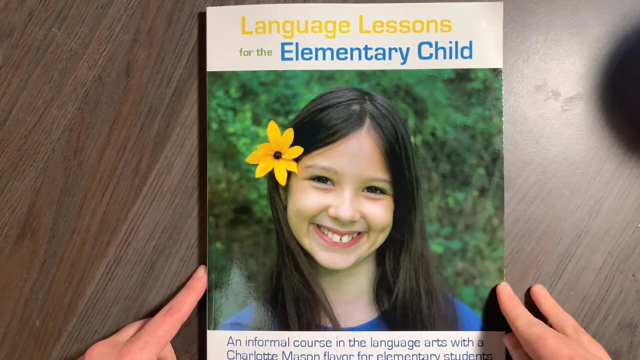 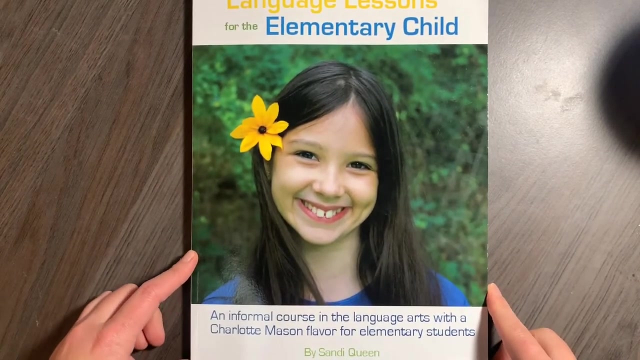 turning 10.. Hi friends, welcome back to Common the Chaos Homeschool. Today I want to do a flip through of language lessons for the elementary child by Saudi Queen. This is from Queen Homeschooling and I'm going to show you right now kind of what the website looks like. Okay, 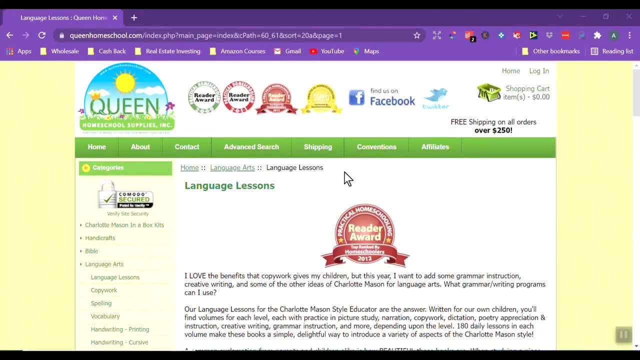 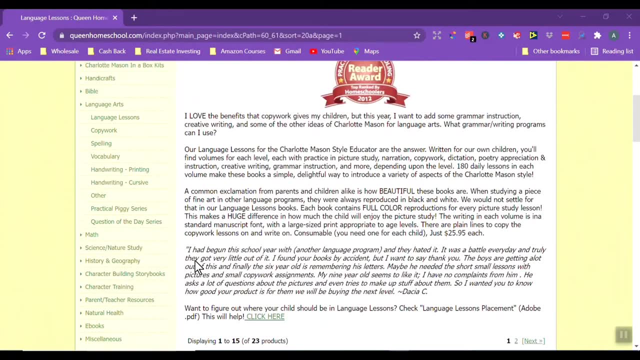 so here I am at queenhomeschoolcom, The language lessons portion. just take a look here on the side they have a wide variety of Charlotte Mason curriculum. So I just wanted to let you know about this in case you've never heard about it, because I've heard a little bit about it, but not much. So just a place to 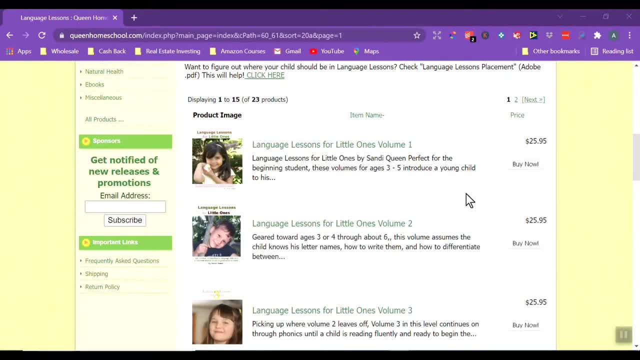 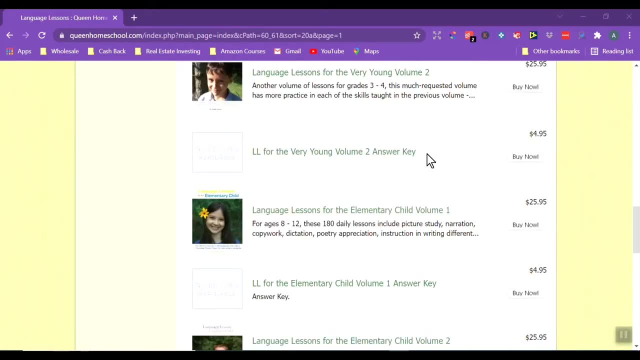 consider if you're Charlotte Mason style, And then down here, so starting very young, they have some language lessons for little ones, language lessons for the very young. And then here we are, here the one I'm doing, the review on language lessons for the elementary child. 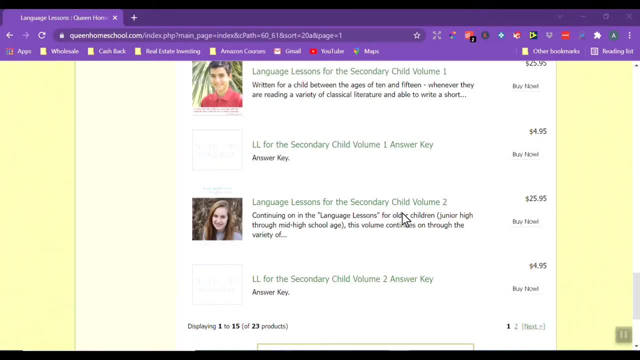 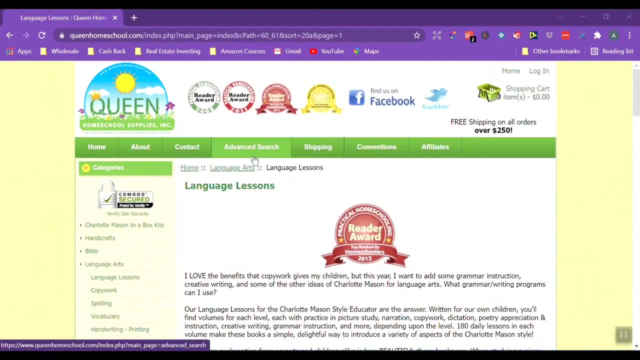 And then they go to secondary child And then on the next page they have more for high school, going through grammar essay writing and then research paper writing. So just another option for you to look at here. So this is language lessons for the elementary child And it's good. 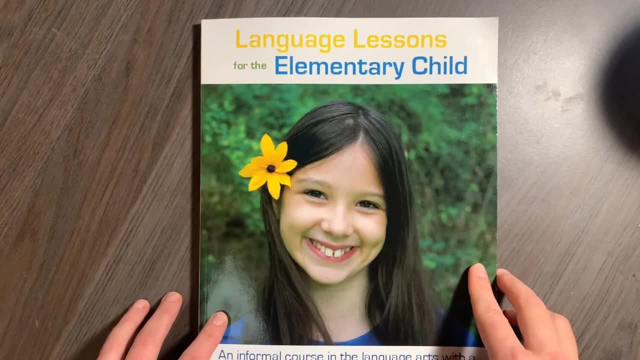 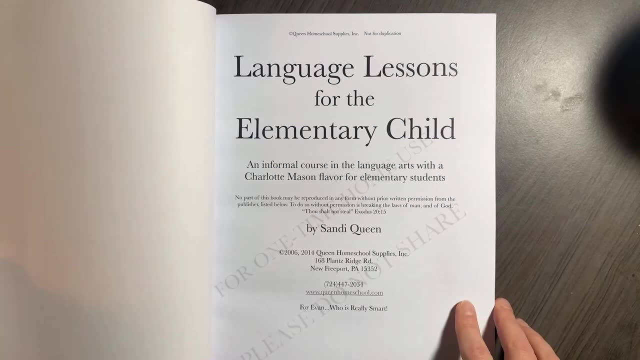 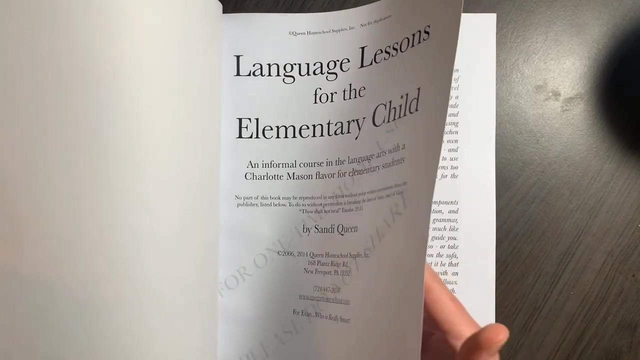 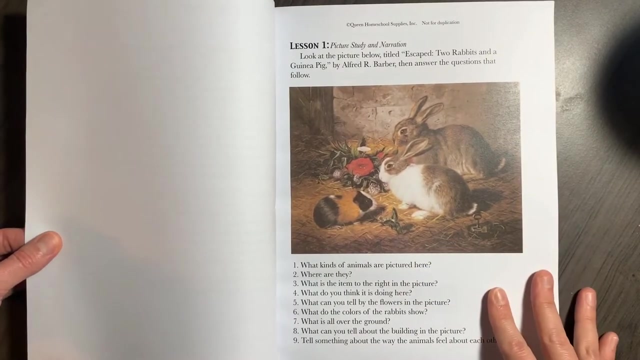 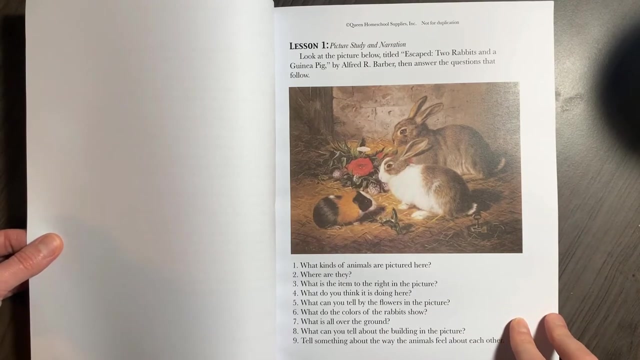 for about probably 8,, 9,, 10,, 11, or 12, depending on their level of language arts. All right, so it's called an informal course in language arts with a Charlotte Mason flavor for elementary students. So what I really like about this curriculum, this language arts curriculum, is that it works very well if you don't want to do a ton of language arts every day or you want to cover all your bases and then maybe do one or two supplemental language arts programs. So it just kind of hits everything. So like for here, lesson one, a picture, study and narration. So they have this beautiful picture here, color picture, and then they have questions that the child can answer. 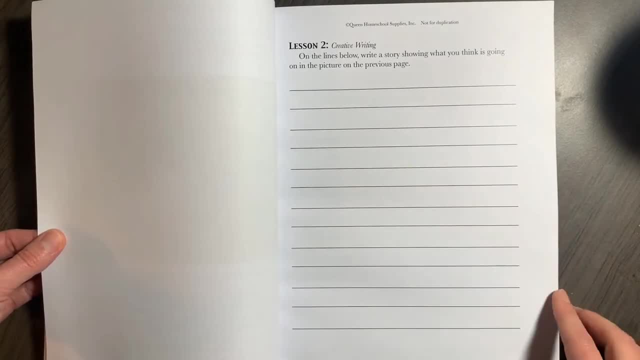 So they have this beautiful picture here, color picture, and then they have questions that the child can answer. Day two: creative writing. It says on the lines below: write a story showing what you think is going on in the picture on the previous page. So some writing. 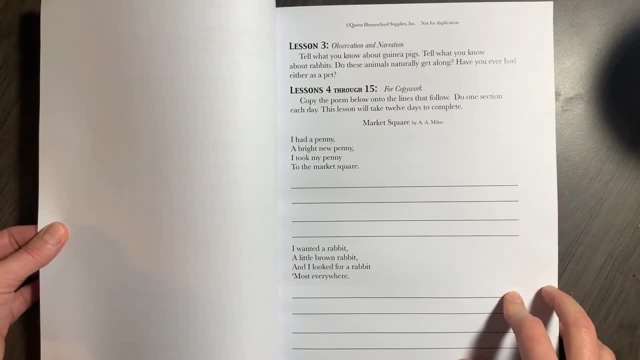 Lesson three: observation and narration. Tell what you know about guinea pigs. Tell what you know about rabbits. Do these animals naturally get along? Have you ever had either as a pet? Here's lessons four through five. copy work. Copy the poem below onto the lines that follow: Do one section each time. 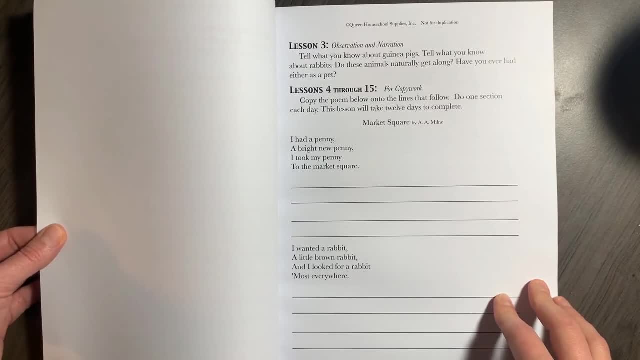 Copy the poem below onto the lines that follow: Do one section each time. Do one section each time day. this lesson will take 12 days to complete, so each day they're just writing this stanza on the lines below. so this goes through several days. that one's a little bit more, but pretty short. 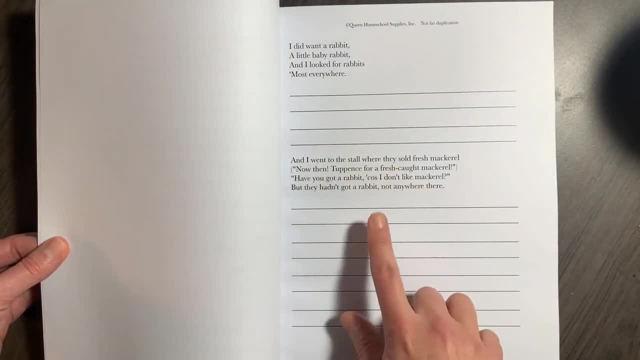 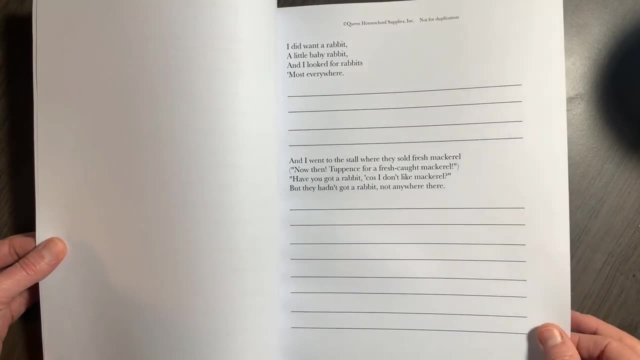 at the beginning and it's about what my boys can handle this is gonna. this would be tough right now, but i am planning on using it closer to the end of the year so hopefully by the time we get to the end of the year they'll be able to handle something like that. so that's several days there. 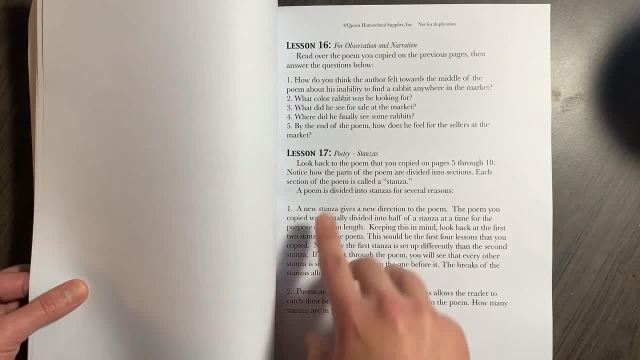 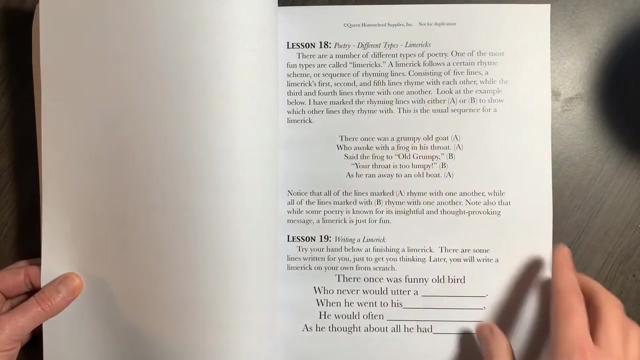 okay then lesson 16 for observation and narration: read over the poem you copied on the previous pages, then answer the following questions. and then there's questions so that they can think about the poetry. then here is talking about stanzas and what. those are different kinds of poetry, limericks. so this they're teaching them: how to write a limerick. 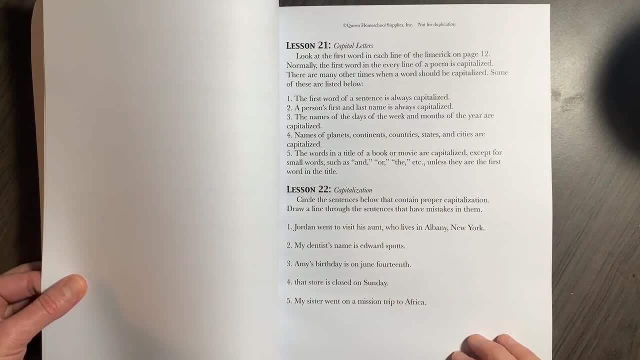 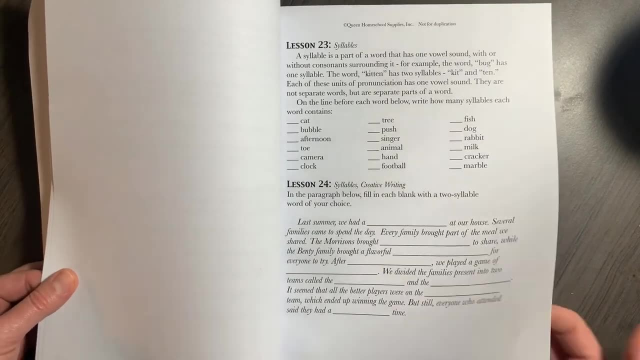 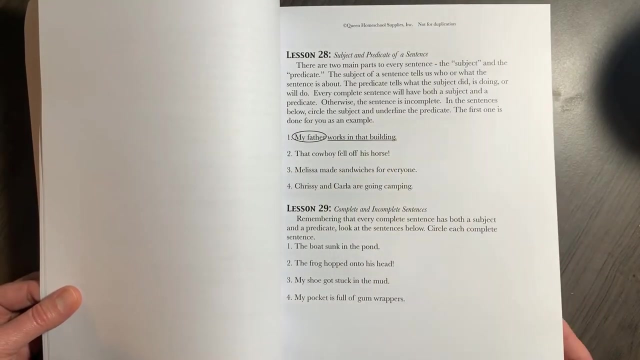 more on limericks. now we have some grammar, capital, owe, capital, letters, capitals, then some 표 or caps, but ch変hhh, capitalization syllables. syllables in creative writing. So, as you can see, they go through there's haikus, they go through a bunch of different things in language arts, but they're. 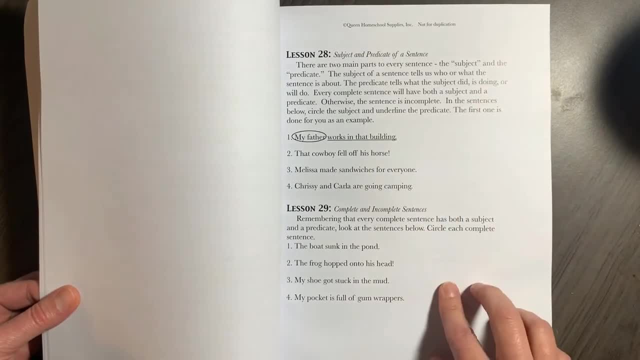 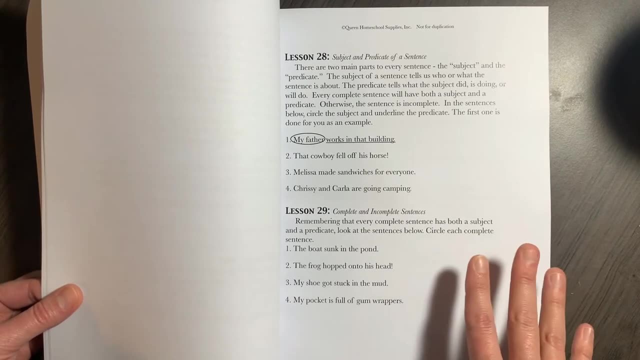 very short lessons. I actually feel like I could probably do two lessons a day with my boys. I think that wouldn't be too much. There are 180 lessons in this curriculum. I would definitely supplement for my boys, depending on which child. I have one child who really needs to work on. 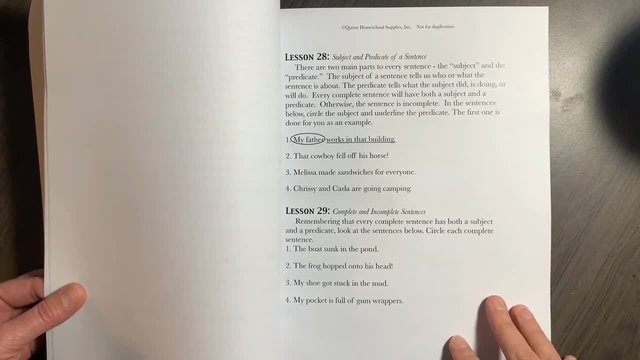 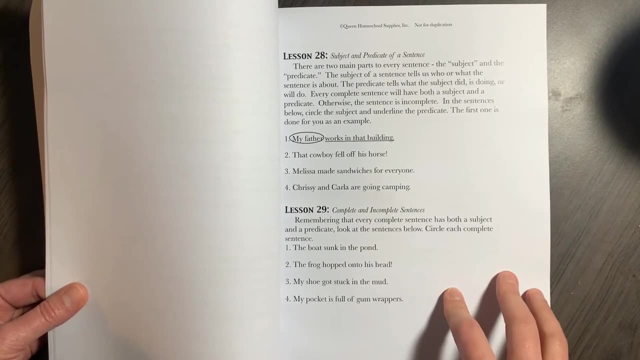 spelling. So he would have a spelling curriculum and it would be very easy for him to do the spelling curriculum and this in a day and not be overwhelmed with language arts, Whereas my other son, he, doesn't need help with spelling, He just picks things up more quickly. So this would just 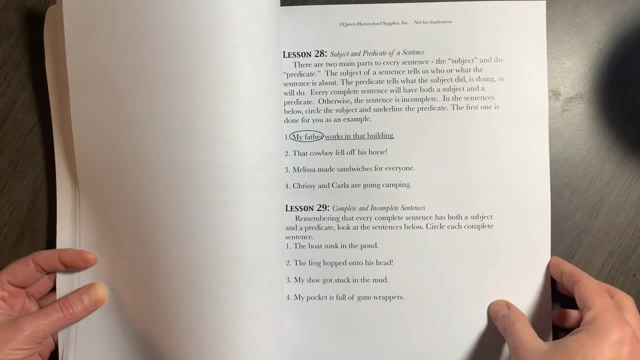 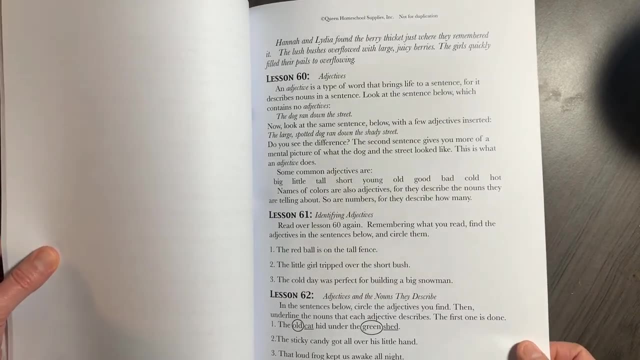 be perfect for him, All right. So I'm going to just flip kind of more a few pages at a time, just so you can see what happens in the middle here. So we're talking about adjectives, identifying adjectives, adjectives and nouns that they describe. another picture study. 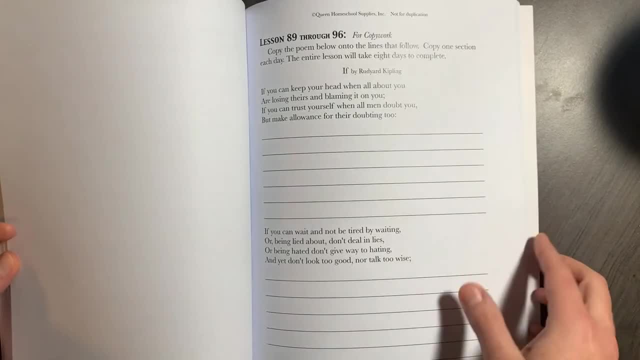 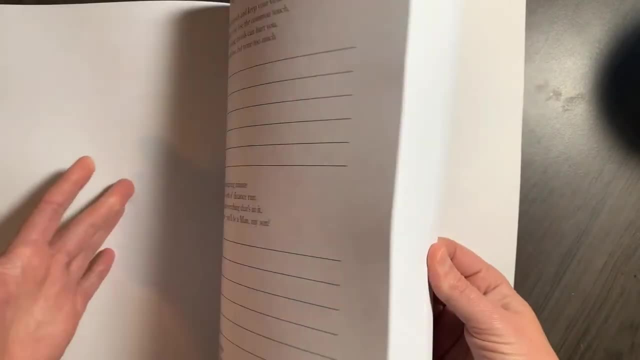 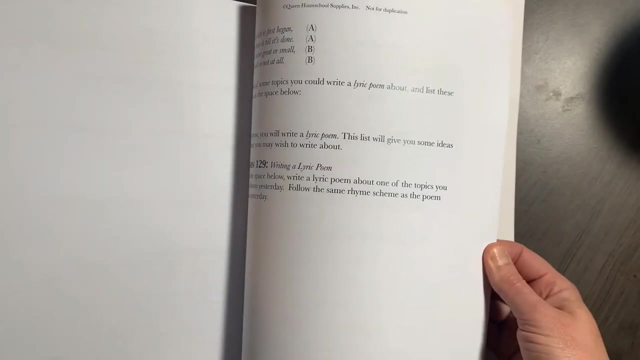 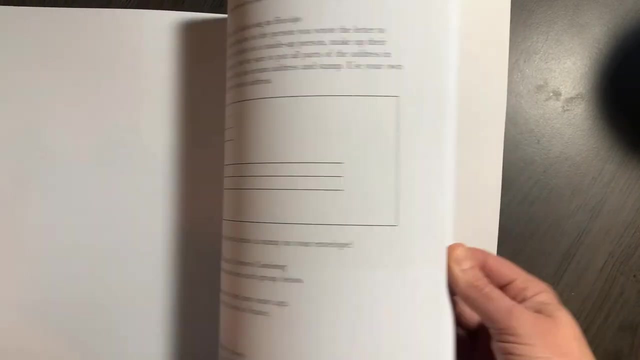 Okay, Lesson 80,, 89, more copy work. Okay, So more copy work. You can see that the copy work is definitely getting longer towards the end of this book. Contractions, narration, Yeah. So I really feel like this is a really great example of a Charlotte Mason type of language arts, I think. 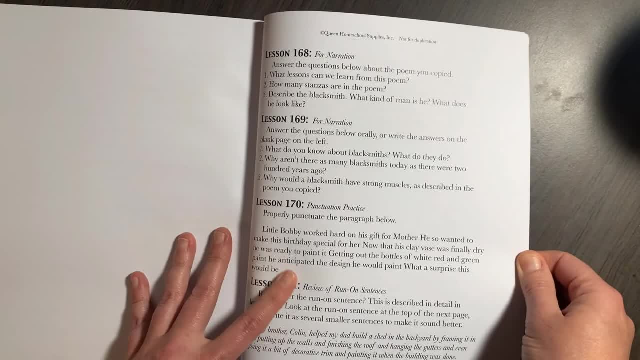 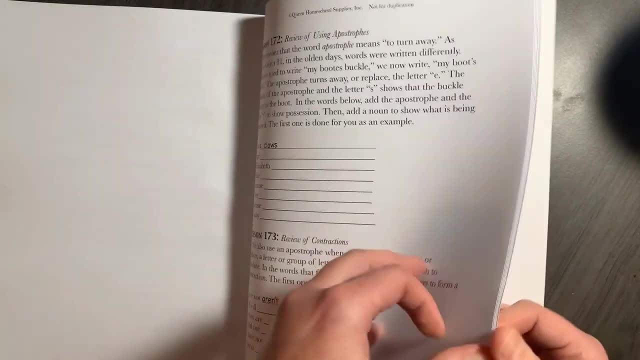 it will be easy for my boys to do- I don't, but I think they'll also be learning. So I'm always very careful, especially with my boys, to just not give them too much, because they can get overwhelmed with the amount of work. All right, So that is the first in the elementary. 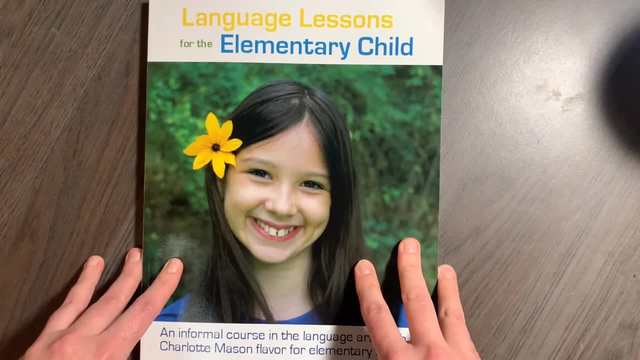 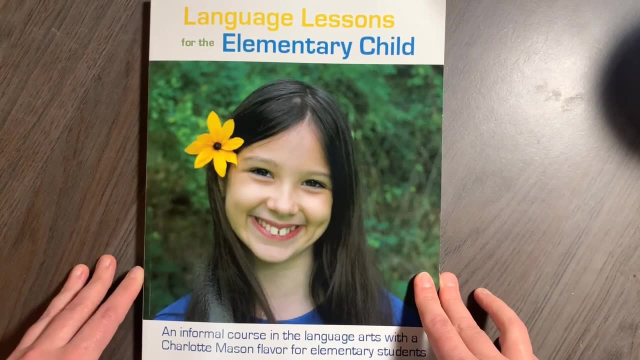 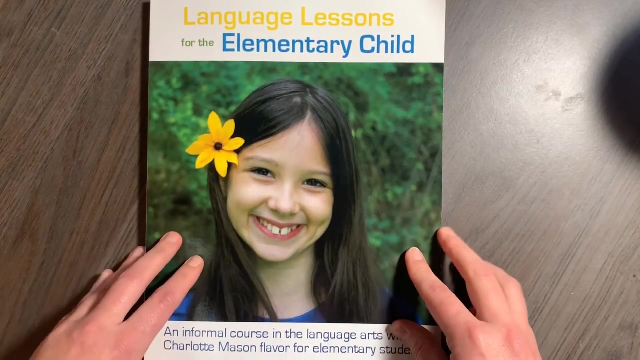 child. They have a lot of books, as you saw on the website, a lot of levels, So you would just need to look and see what level works for you. I'm very happy with this. One thing to note is it is a consumable product, So you are not allowed to make photocopies. So 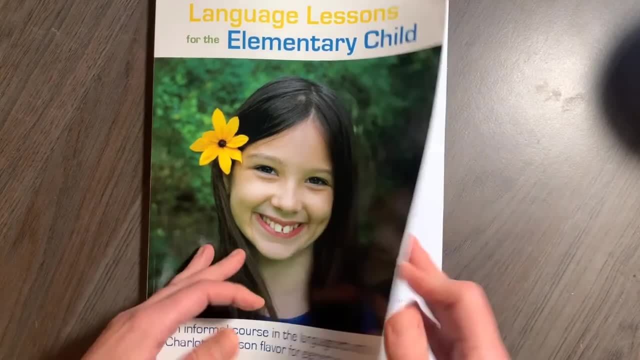 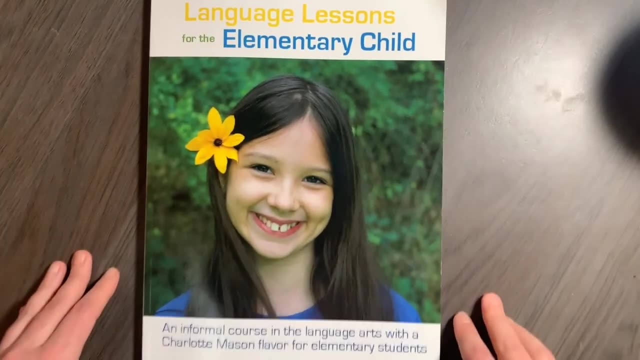 I will have to buy one more for my other son when we do use this- but I do, I- I really I think it's well laid out and I think the lessons are very thorough, and I'm excited about using this whenever my boys are finished. what they're working on right now, All right. So thank you. 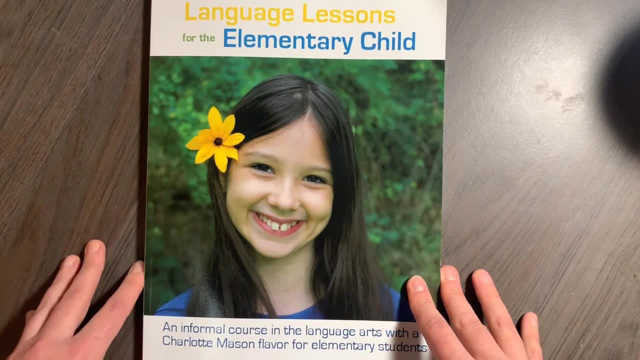 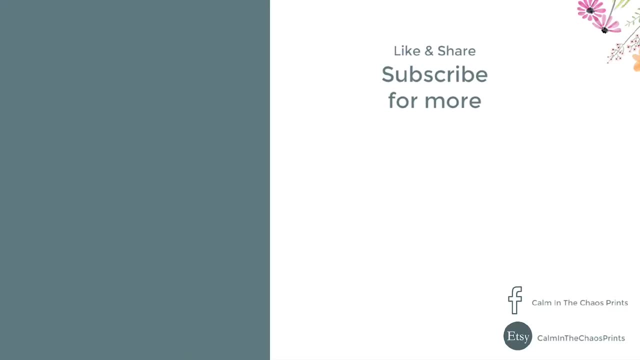 for watching. Please like and subscribe If you'd like to see more flip throughs of the different curriculum that I'll be using or that I have used. Thanks, Bye-bye, Bye-bye.